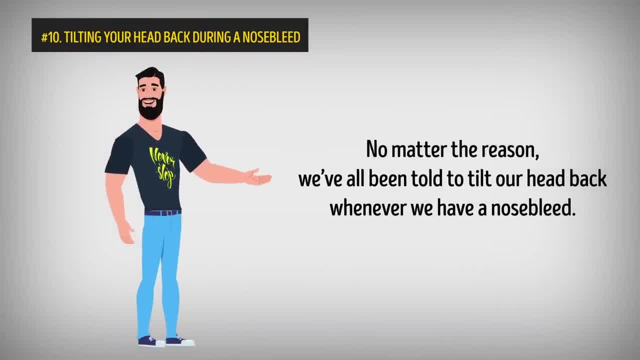 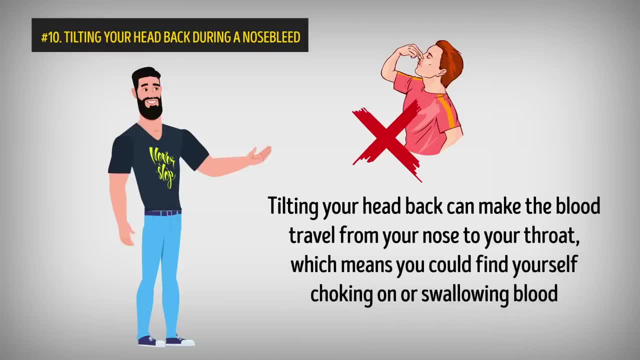 No matter what the reason, we've all been told to tilt our head back whenever we have a nosebleed, But it's high time to ditch this old habit. Tilting your head back can make the blood travel from your nose to your throat. 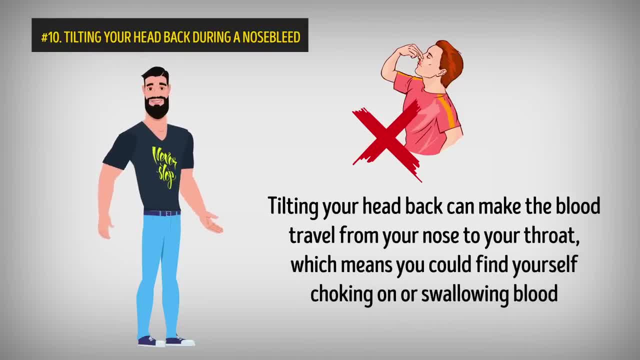 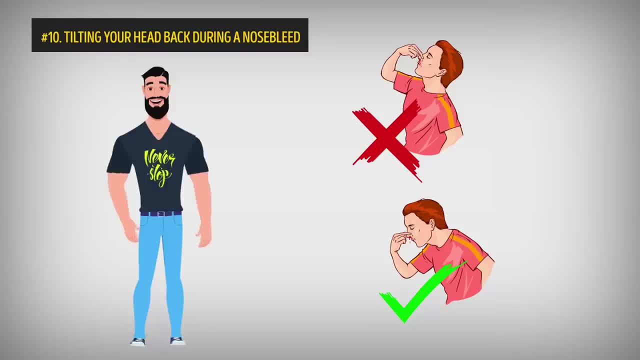 which means you could find yourself choking on or swallowing blood. The best thing to do instead is to apply steady pressure to the bridge of your nose for at least 20 minutes. You'll have to breathe through your mouth this whole time, but you'll safely stop the bleeding. 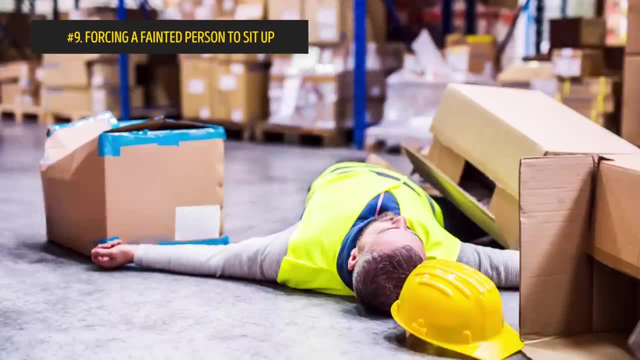 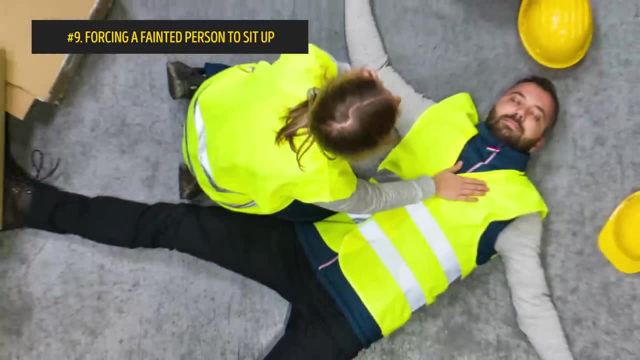 9. Number 9. Forcing a Fainted Person to Sit Up. When someone faints, our immediate course of action is to try to sit them up, especially when shaking them doesn't seem to be helping. Instead of all that, always start by checking their breathing and pulse. 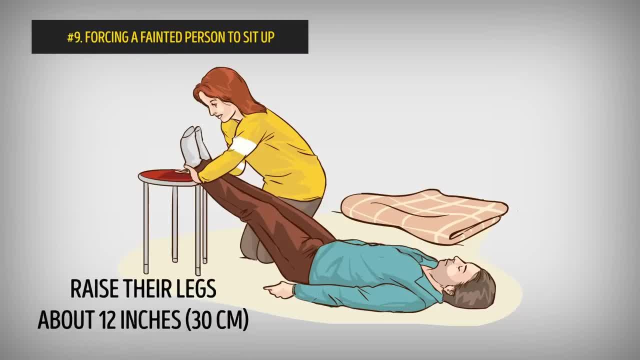 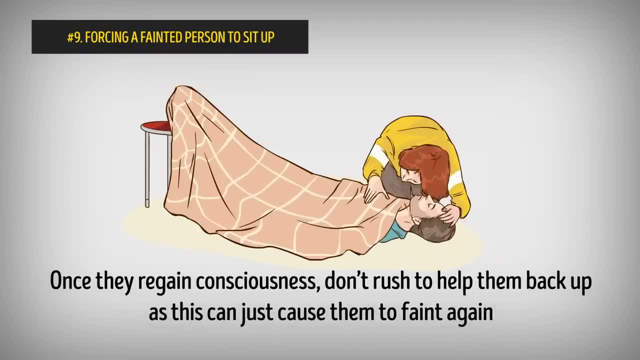 If that's all good, leave them on the ground, but raise their legs about 12 inches off the floor. Loosen any restrictive clothing as well. Once they regain consciousness, don't rush to help them back up, as this can just cause them to faint again. 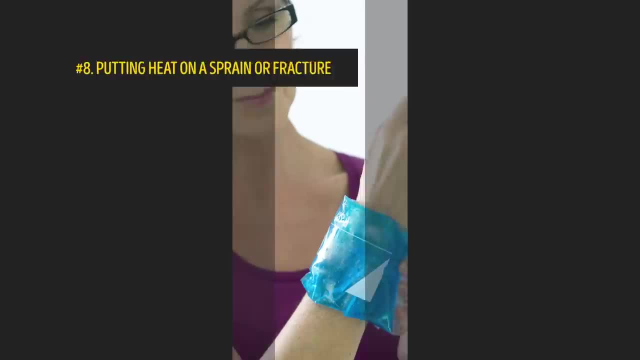 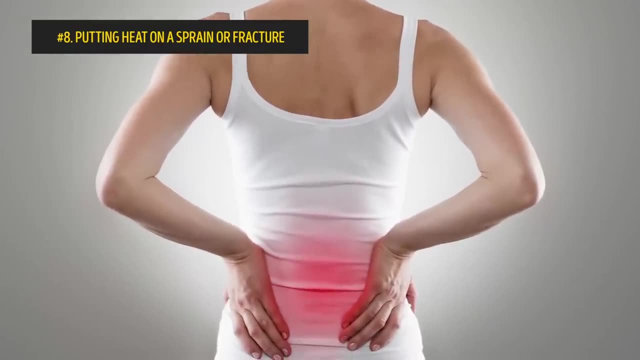 Number 8. Putting Heat on a Sprain or Fracture. Ice should be used for acute situations like suddenly spraining your ankle. Heat is for chronic conditions like back pain. Heat on a sprain or fracture only increases blood flow and leads to more swelling. 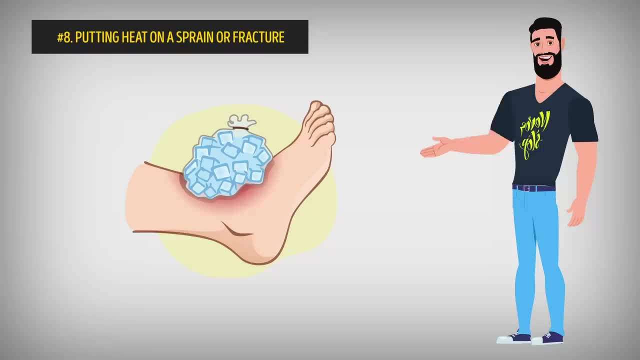 The way to go for these types of injuries is always to ice it at first. The ice will help reduce any swelling, bruising and muscle spasms. Never place an ice pack directly on your skin and be sure to leave it on for at least 20 minutes. 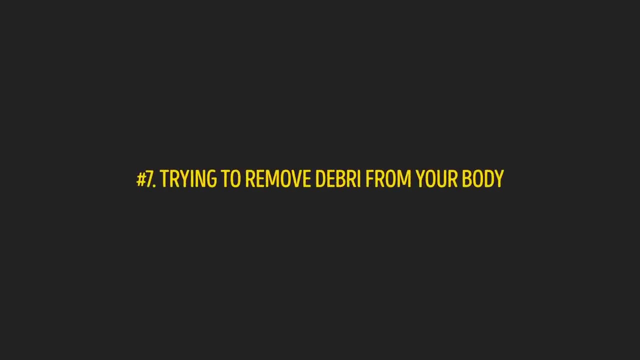 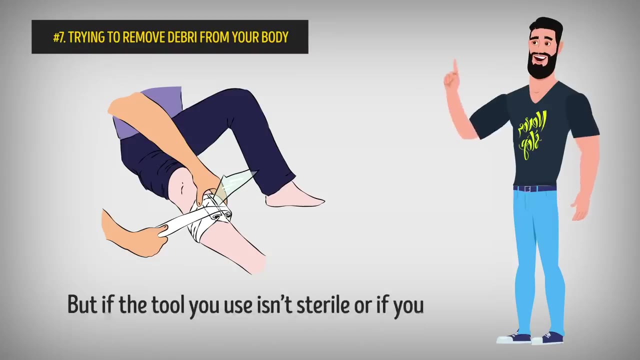 Number 7. Trying to Remove Debris from Your Body. If you step on some glass, for example, your gut reaction will be to pull those shards out of your skin yourself. But if the tool you use isn't sterile or if you underestimate how deep the wound is, 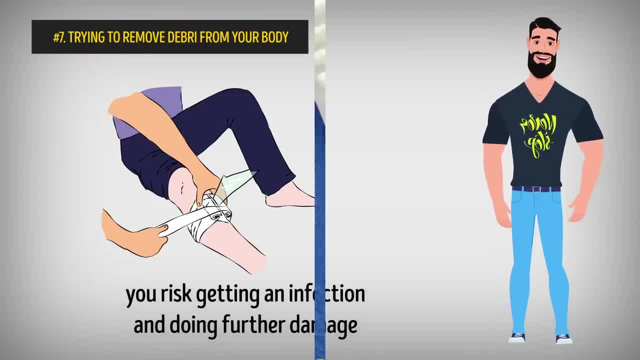 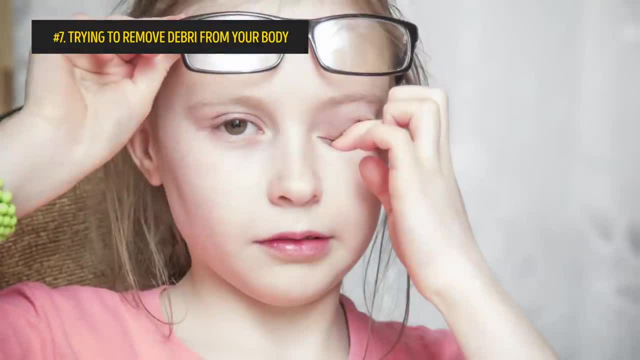 you risk getting an infection and doing further damage, So make sure you're using a clean, sterile tool or leave it in the hands of professionals. When it comes to debris in your eye, it's best to close your eye, put a piece of gauze over it and then put it on your skin. 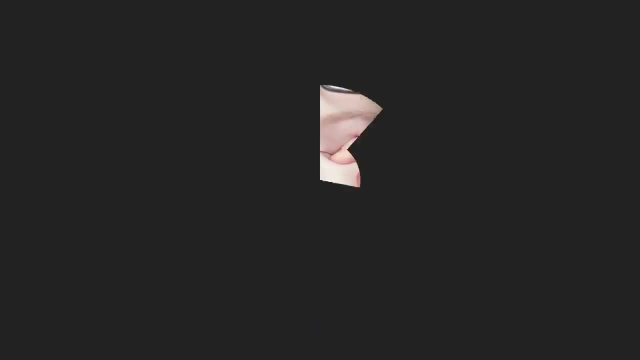 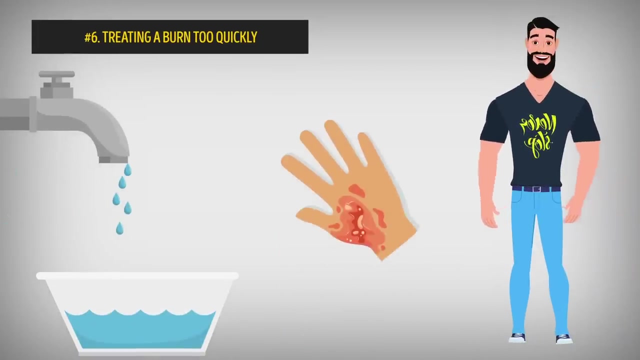 Put a piece of gauze over it and head to the hospital Number 6.. Treating a Burn Too Quickly. The first step to treating a burn is to run it under cool water, But a common mistake is to just do it for a few seconds, or a couple of minutes tops. 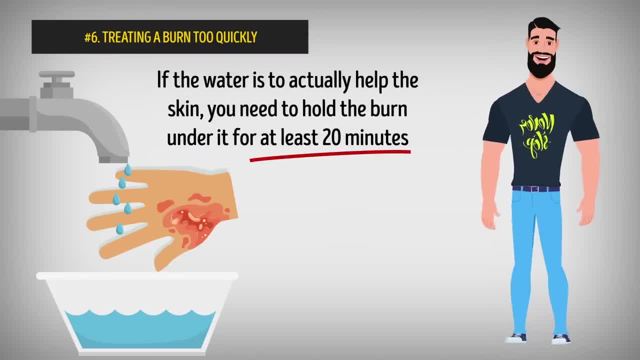 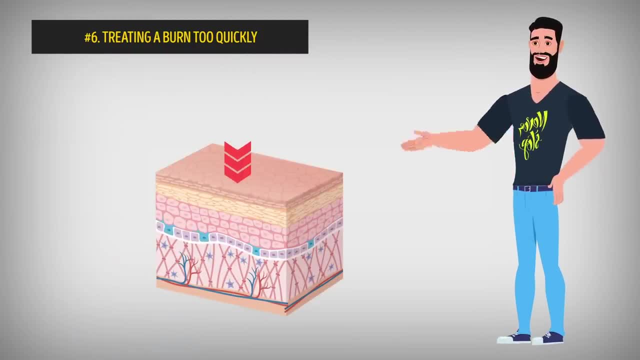 If the water is to actually help the skin, you need to hold the burn under it for at least 20 minutes. The heat from the burn can go deep across several layers of skin, So even if your skin is cool on the surface, it can still be trapped underneath, which is why you need to expose it to cool water for such a long time. 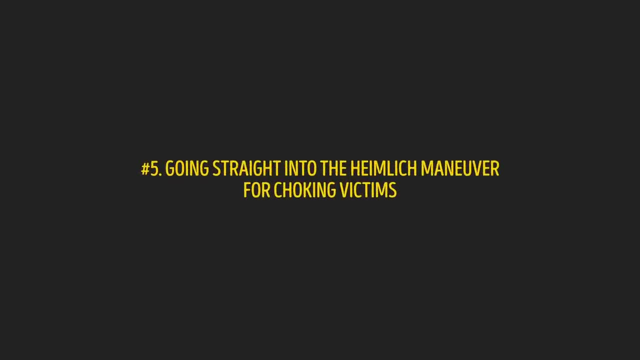 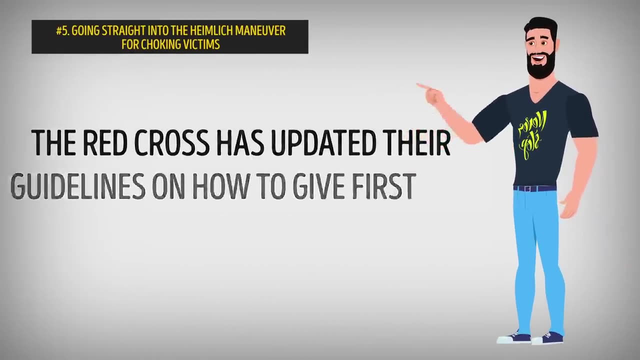 Number 5. Going Straight into the Heimlich Maneuver for Choking Victims. The Red Cross has updated their guidelines on how to give first aid to choking victims. So, instead of going straight for the Heimlich Maneuver, here's what you're supposed to do instead. 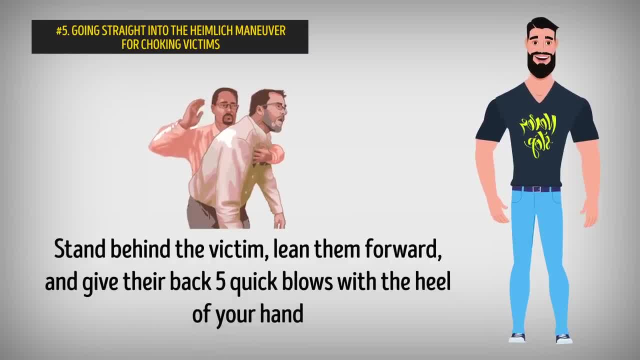 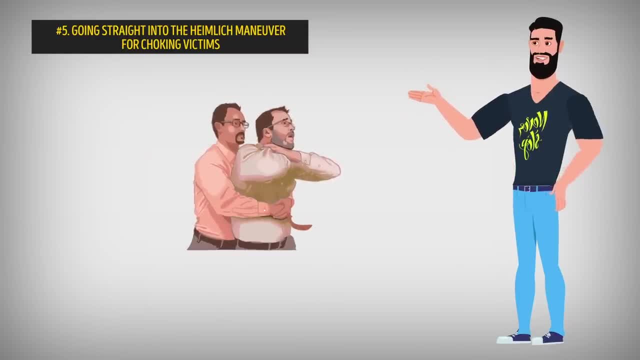 Stand behind the victim, lean them forward and give their back five quick blows with the heel of your hand. Only if that doesn't work, you can't do it. But if that doesn't work at first, can you follow it up with the Heimlich Maneuver. 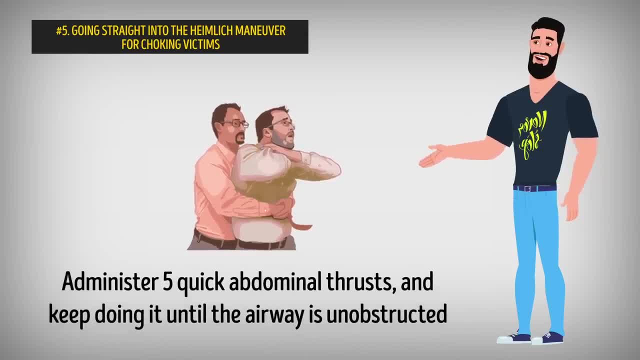 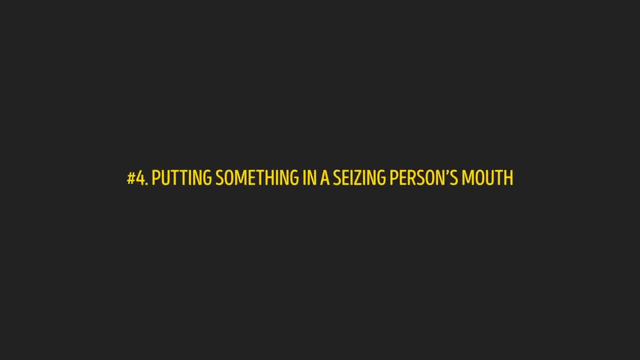 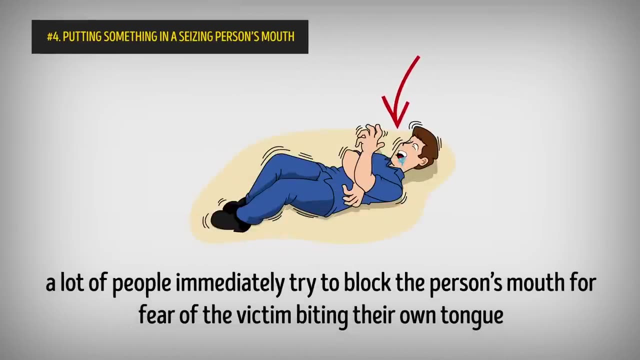 Administer five quick abdominal thrusts and keep doing it until the airway is unobstructed. Number 4. Putting Something in a Seizing Person's Mouth. In a panic-induced state at seeing someone having a seizure, a lot of people immediately try to block the person's mouth for fear of the victim biting their own tongue. 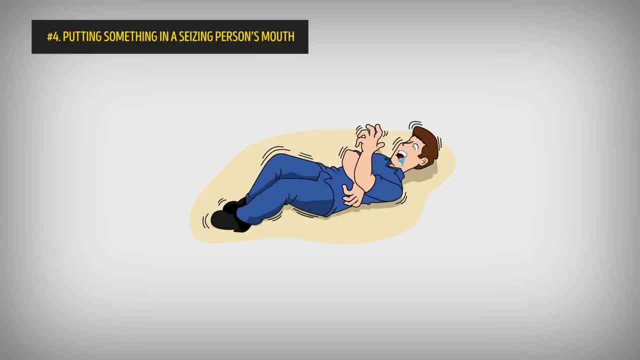 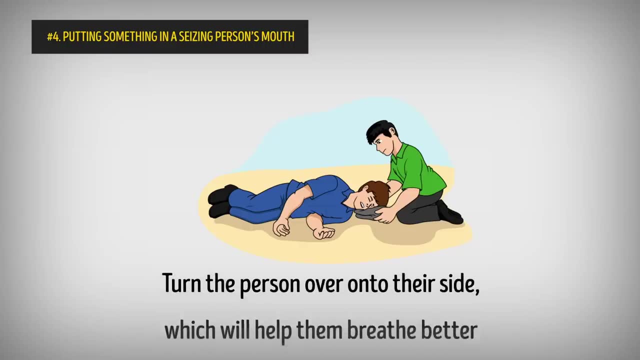 This is actually dangerous for the victim and for the person trying to help. Another mistake is trying to restrain the person. The thing to do instead is to turn the person over onto their side, which will help them breathe easier, Also clear out the area of any dangerous objects the victim could hurt themselves on. 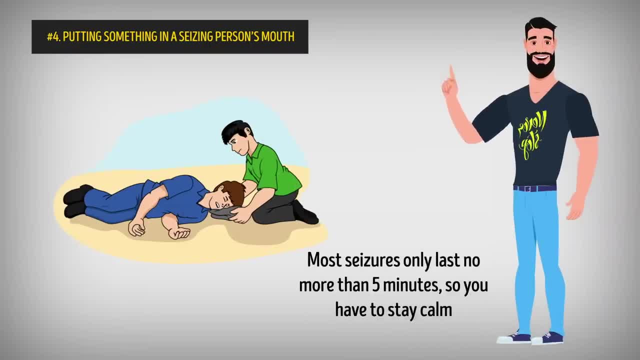 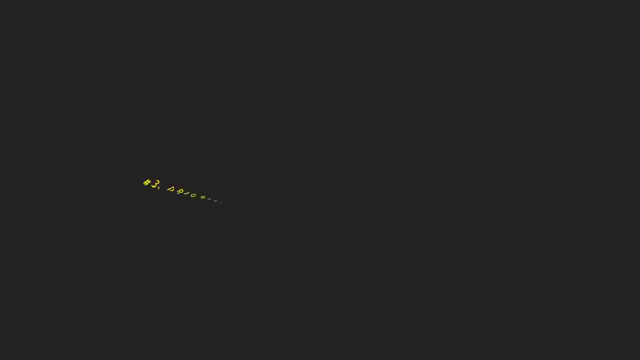 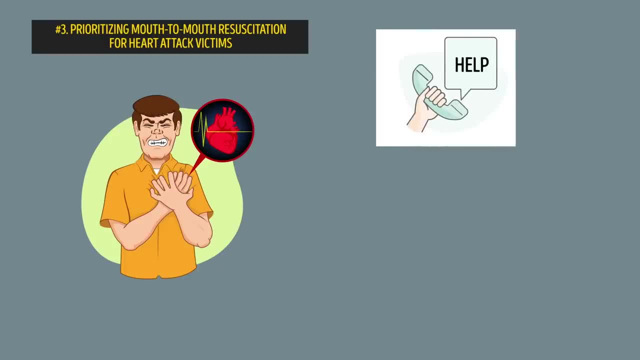 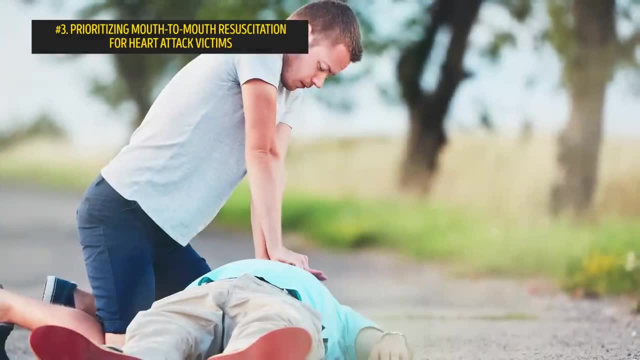 When you have cardiac conditions like a heart attack, the first step is to always dial emergency medical services, Then administer chest compressions or CPR. According to the American Heart Association, CPR can double or even triple the chances of someone's survival. 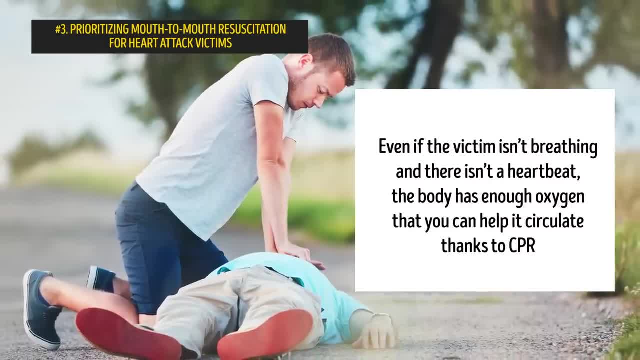 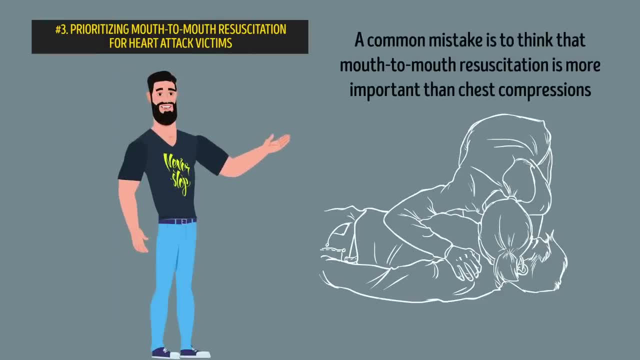 Even if the victim isn't breathing and there isn't a heartbeat, the body has enough oxygen that you can help it circulate thanks to CPR. A common mistake is to think that mouth-to-mouth resuscitation is more important than chest compressions. 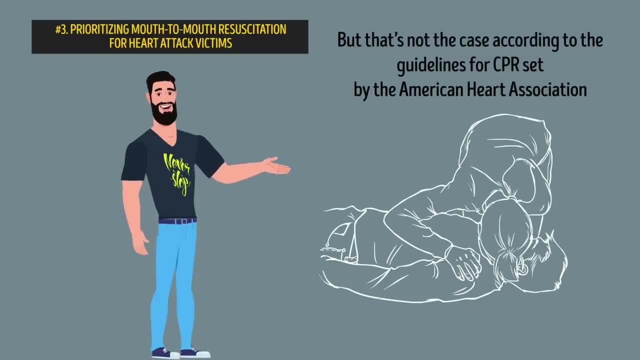 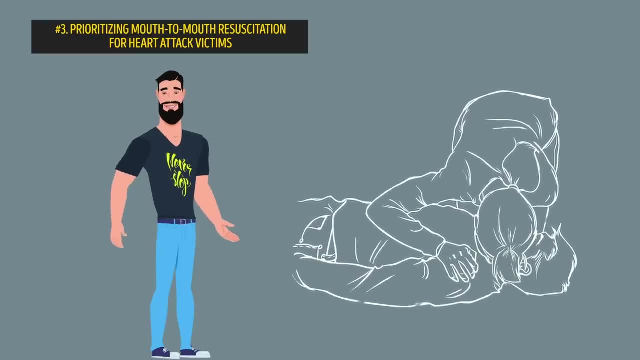 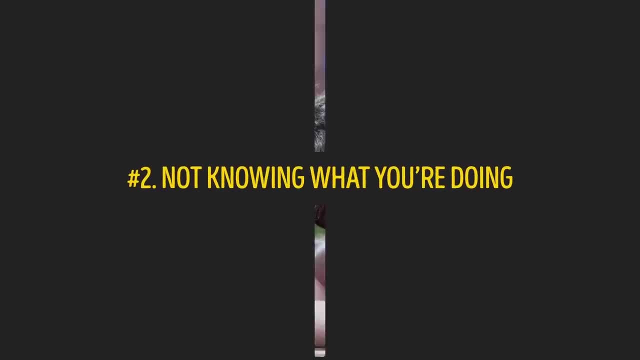 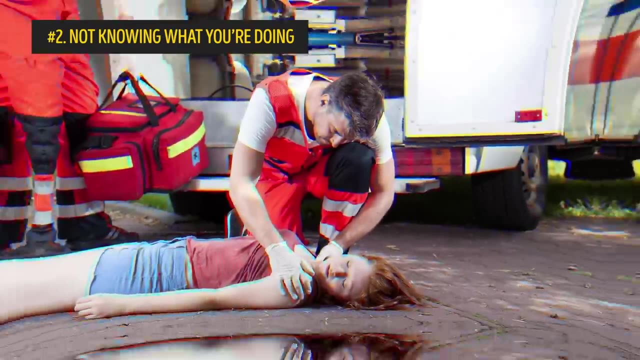 Number two: not knowing what you're doing. Again, good Samaritans mean well when it comes to helping someone in an emergency situation, But if you don't know how to, for instance, administer CPR or the Heimlich maneuver correctly, 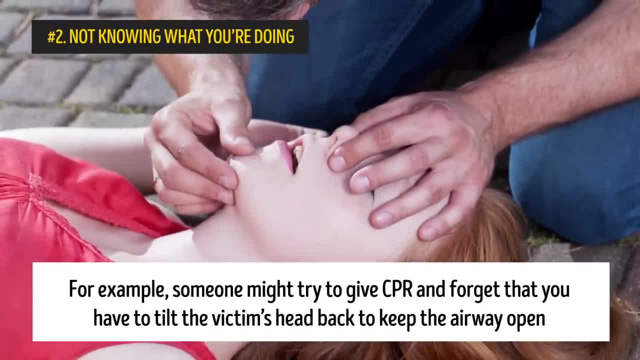 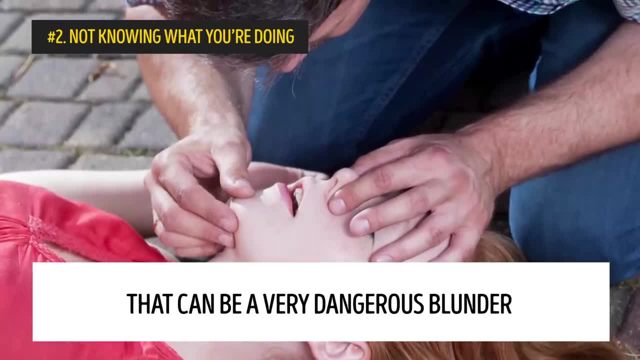 you can end up doing more harm than good. For example, someone might try to give CPR and forget that you have to tilt the victim's head back to keep the airway open. That can be a very dangerous blunder. That's why the first line of action in all serious first aid situations is to call for help. 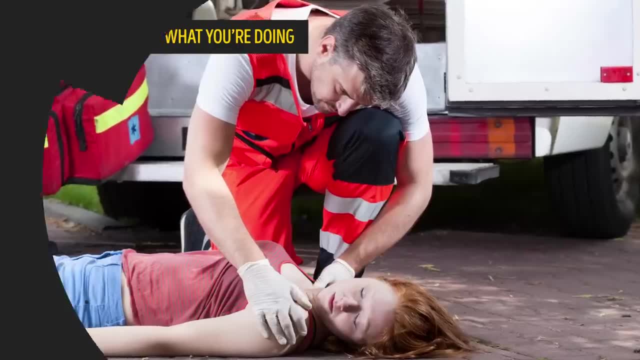 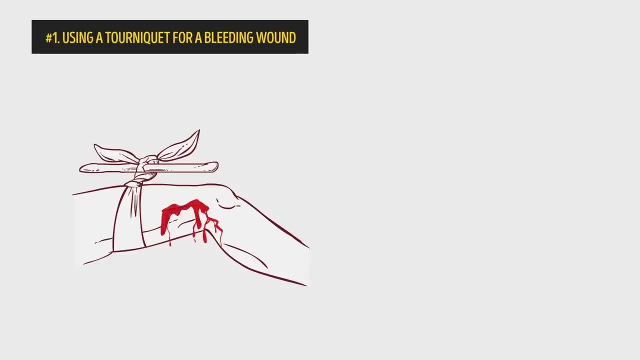 and let a professional guide you through what you need to do. Number one: using a tourniquet for a bleeding wound. Yes, tourniquets can stop a person from bleeding, but it's not a fix-all solution for any type of wound. 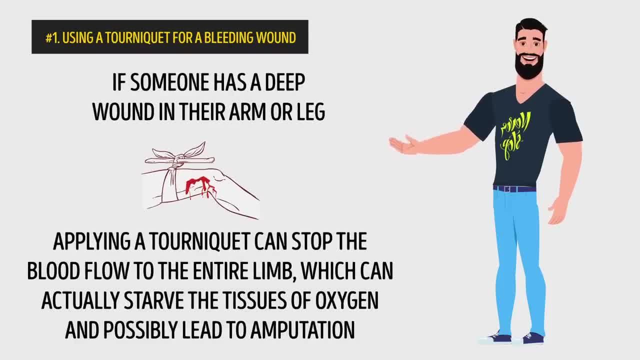 If someone has a deep wound in their arm or leg, applying a tourniquet can stop the blood flow to the entire limb, which can actually starve the tissues of oxygen and possibly lead to amputation. Using a tourniquet should never be a problem.